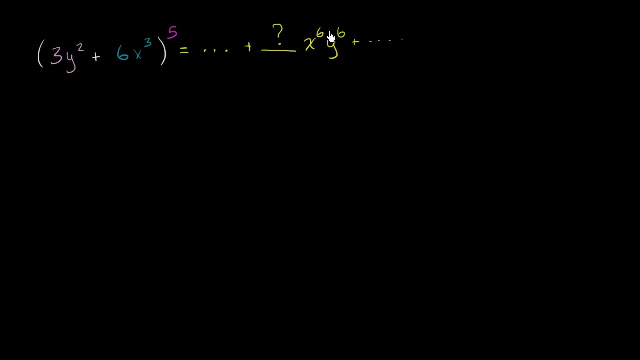 this to be a little bit confusing. I'm only raising it to the fifth power. How do I get x to the sixth, y to the sixth? But then, when you look at the actual terms of the binomial, it starts to jump out at you. 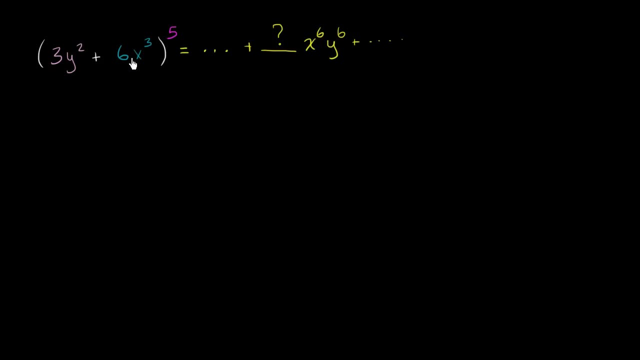 OK, I have a y squared term, I have an x to the third term, So when I raise these two powers I could have powers higher than the fifth power. But actually think about it: Which of these terms has the x to the sixth? y to the sixth? 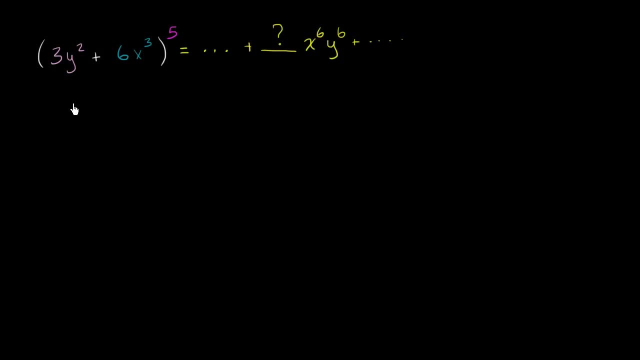 Let's just look at the pattern in the actual expansion, without even thinking about its coefficients- And we've seen this multiple times before- where you could take your first term in your binomial and you can start it off. It's going to start off at the power. 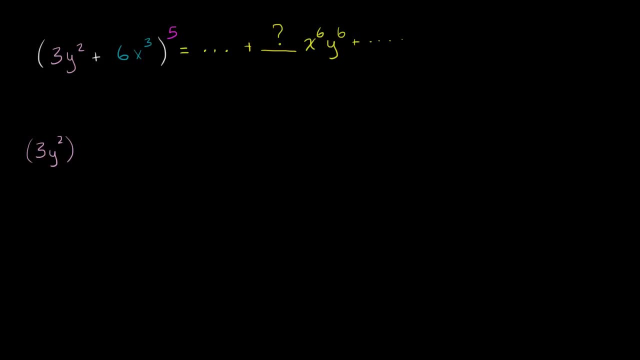 we're taking the whole binomial to, And then in each term it's going to have a lower and lower power. So let me actually just copy and paste this. So this is going to be so copy, And so that's first term. second term. 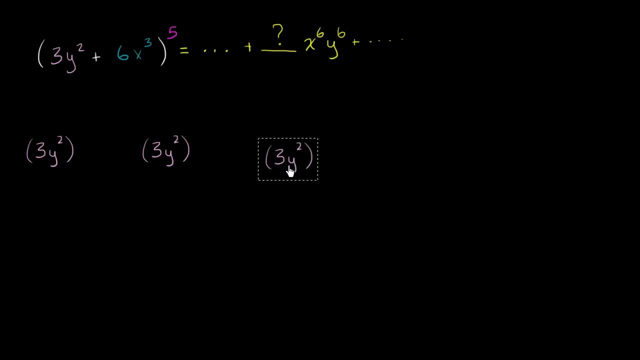 Let me make sure I have enough space here. Second term, third term, fourth term, fifth term And sixth term. this is going to have six terms to it. You always have one more term than the exponent, And then, actually, before I throw the exponents on it, 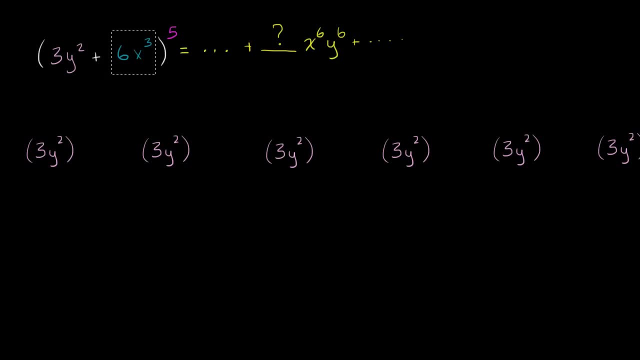 let's focus on the second term. So the second term. actually, I'll write it like this: So the second term is times six x to the third. Let me copy and paste that. Whoops, So let me copy and paste that. 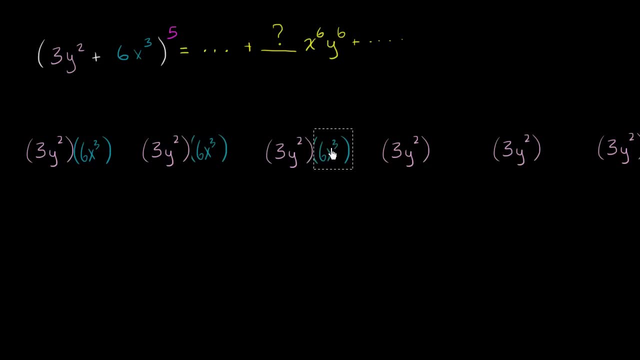 So we're going to put that there, that there and that there and that there, And then over, actually off your screen. I wrote it over there, So we'll see if we have to go there, And then let's put the exponents. 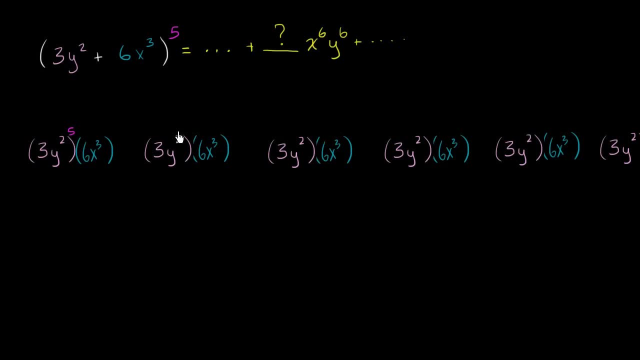 So this exponent, this is going to be the fifth power, fourth power, third power, second power, first power and zeroth power. And for the blue expression for six, x to the third, this is going to be the zeroth power, first power. 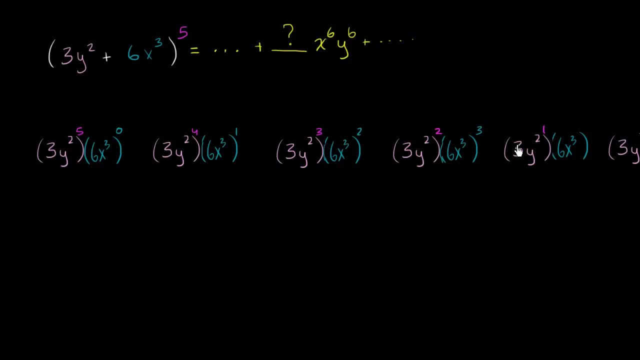 second power, third power, fourth power, And then we're going to go there. All right. So we're going to have the fifth power right over here And, of course, they're each going to have coefficients in front of them. They're each going to have coefficients in front of them. 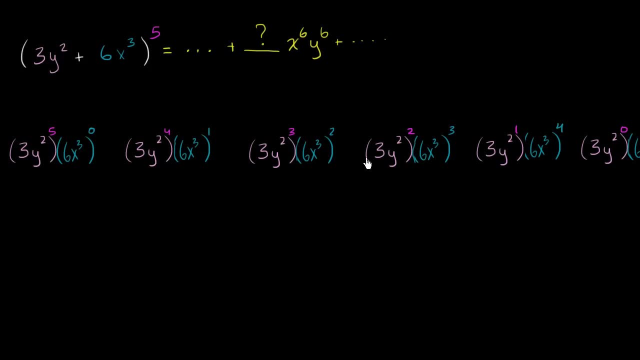 So there's going to be a coefficient in front of this one, in front of this one, in front of this one, And then we add them all together, But which of these terms is the one that we're talking about? Has x to the sixth, y to the sixth. 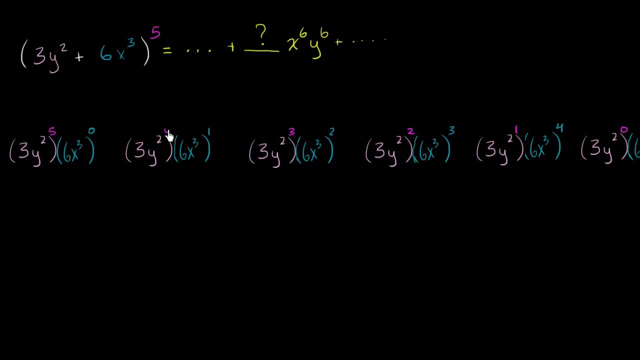 So here we have x. if we take y squared to the fourth, that's going to be y to the eighth. So that's not it. If we go here, we have y squared to the third, to the third power, That's y to the sixth. 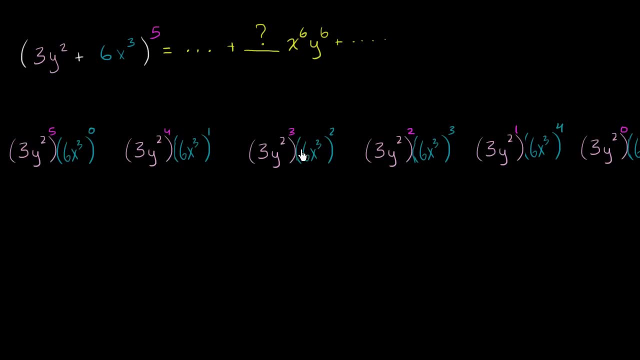 And here you have x to the third, squared, That's x to the sixth. So what we really want to think about is what is the coefficient in front of this term going to be? Essentially, if you put it in this way, it's going to be the third term that we actually care about. 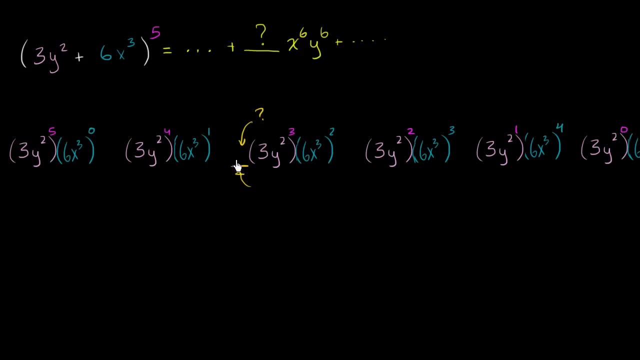 So what is this coefficient going to be? Now, we have to be clear. This coefficient, whatever we put here that we can use the binomial theorem to figure out, isn't going to be this, This thing that we have to, I guess. 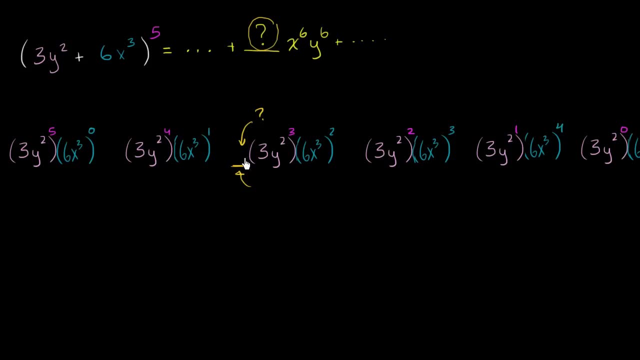 our actual solution to the problem that we posed is going to be the product of this coefficient and whatever other coefficients we have over here, Because we're going to have 3 to the third power, 6 squared, So we're going to have to figure out what that is. 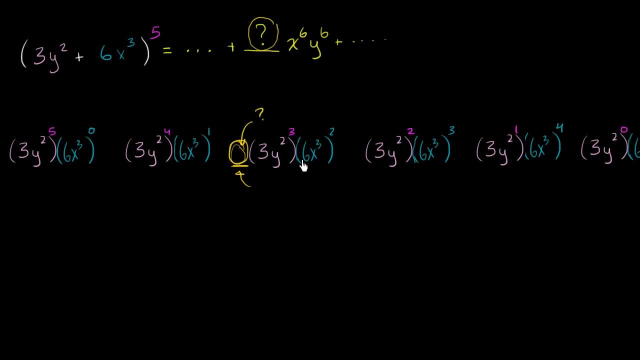 But let's first just figure out what this term looks like, this term in the expansion, what this yellow part actually is. And there's a couple of ways we could do that. We could use Pascal's triangle, or we could use combinatorics. 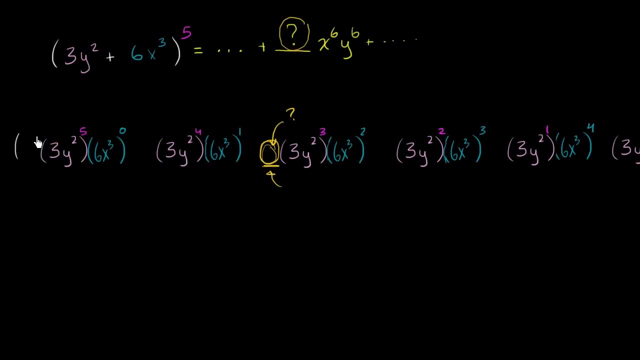 If we use combinatorics, we know that the coefficient over here this is going to be 5 choose 0. This is going to be the coefficient over here is going to be 5 choose 1.. And we've seen this multiple times. 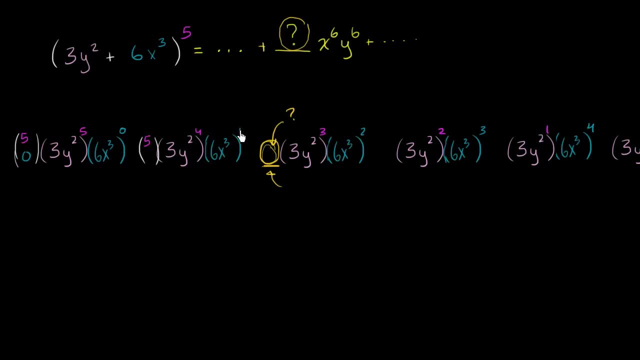 You could view it as essentially the exponent choose the top. the 5 is the exponent that we're raising the whole binomial to, And then when we say choose this number, that's the exponent on the second term. I guess you could say: 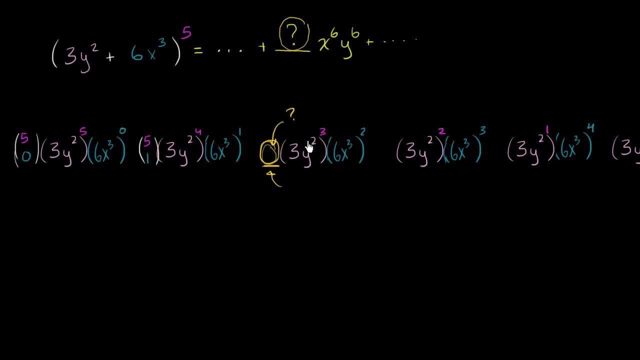 So this would be 5 choose 1.. And this one over here, the coefficient, this thing in yellow, this is going to be 5 choose 2.. Now, what is 5 choose 2?? Well, that's equal to 5 factorial over 2 factorial. 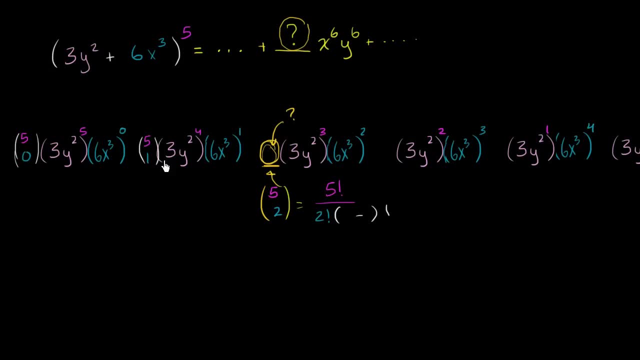 times 5- choose 2.. 5- choose 2.. 5- choose 2.. 5 minus 2 factorial. So let me just put that in here: Times 5 minus 2 factorial And this is going to be equal to: let's see. 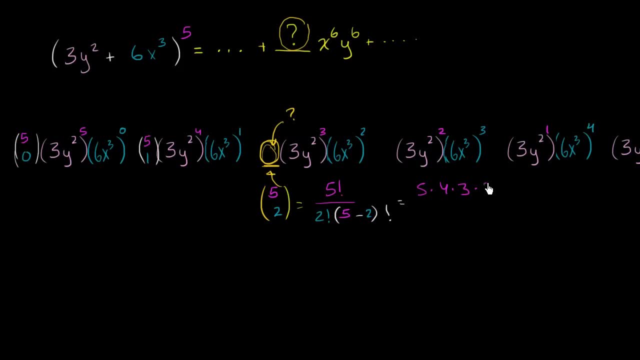 5 factorial is 5 times 4 times 3 times 2.. We could write times 1,, but that won't change the value Over 2 factorial. Actually, let me just write that, just so we make it clear. It is times 1 there. 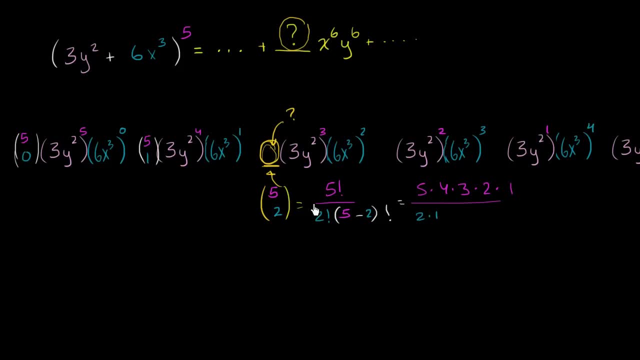 2 factorial is 2 times 1.. And then what we have right over here is 3 factorial, So times 3 times 2 times 1.. So let's see this: 3 could cancel with that 3.. That 2 could cancel with that 2.. 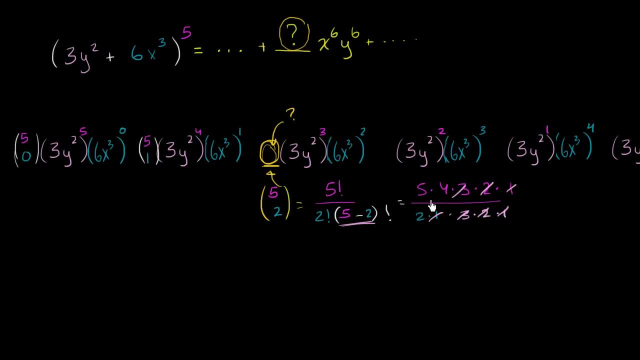 The 1's don't matter, won't change the value. And then 4 divided by 2 is 2.. So that is just 2.. So we're left with: 5 times 2 is equal to 10.. So that's going to be this number right over here. 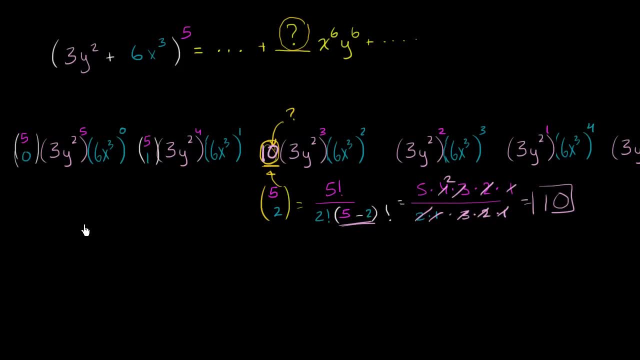 This is going to be a 10.. Now, another way we could have done it is using Pascal's triangle. We could have said: okay, this is the binomial. now, this is when I raise it to the second. power is 1, 2, 1 are the coefficients. 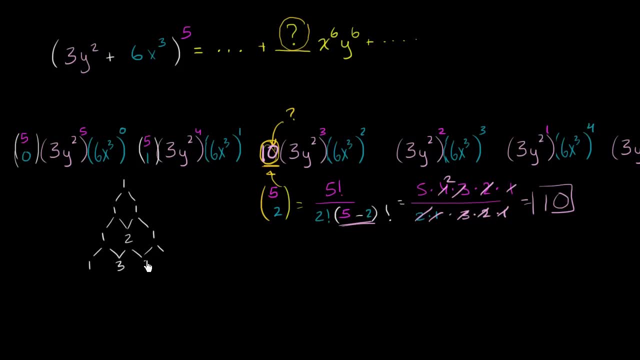 When I raise it to the third power, the coefficients are 1,, 3,, 3,, 1.. When I raise it to the fourth power, the coefficients are 1,, 4,, 6,, 4,, 1.. 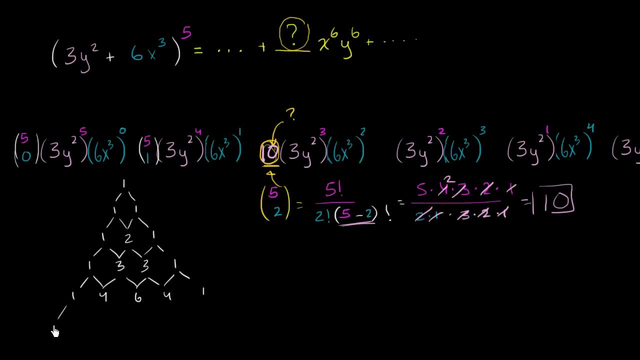 And when I raise it to the fifth power, which is the one we care about, the coefficients are going to be 1,, 5,, 10,, 5, or sorry, 10,, 10,, 5, and 1.. 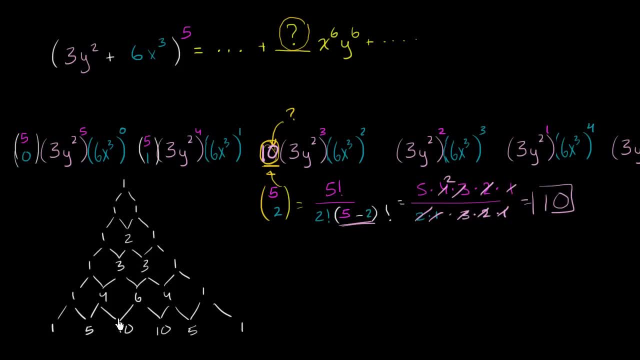 And we know that when we go for this is going to be the third term, So this is going to be the coefficient right over here: 1,, 2,, 3, third term. So either way, we know this is 10,. 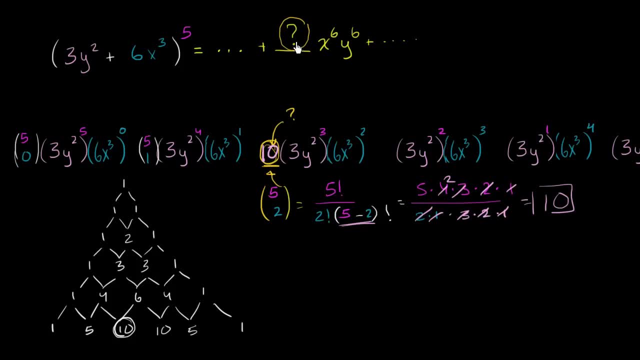 but now let's try to answer our original question. What is this going to be? What are we multiplying times x to the sixth, y to the sixth, And now we just have to essentially rewrite this expression. So it's going to be 10 times 3 to the third power. 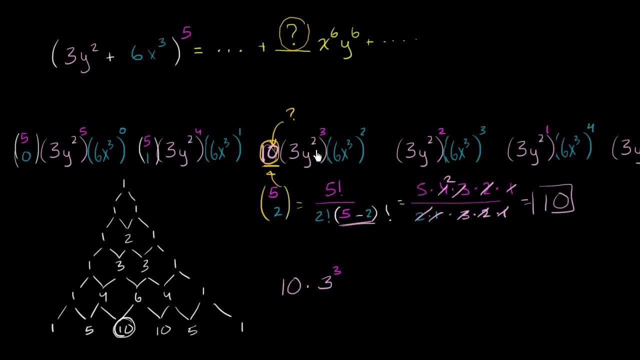 times y squared to the third power, which is y squared to the third power is y to the sixth power times 6 squared. so times 6 squared times x to the third squared, which that's x to the three times two. 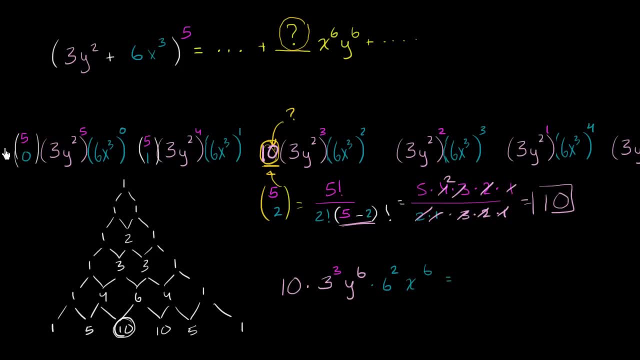 or x to the sixth, And so this is going to be equal to: let's see, it's going to be 10, times times 27, times 36, times 36th, and then we have, of course, our x to the 6th and y to the 6th. 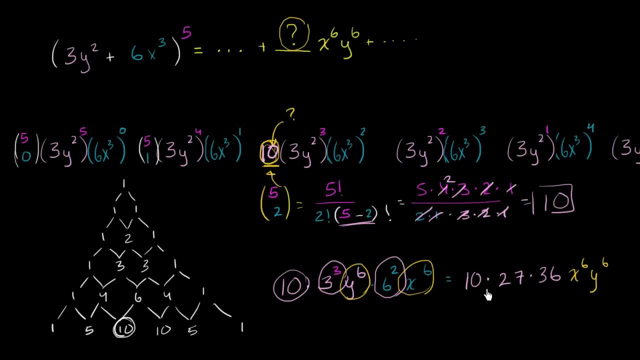 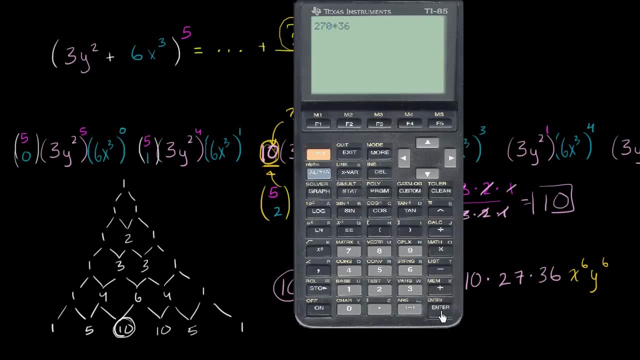 So this is going to be essentially, let's see 270 times 36, so let's see, let's get a calculator out, 270,. I could have done it by hand, but I'll just do this for the sake of time. times 36 is 9720.. 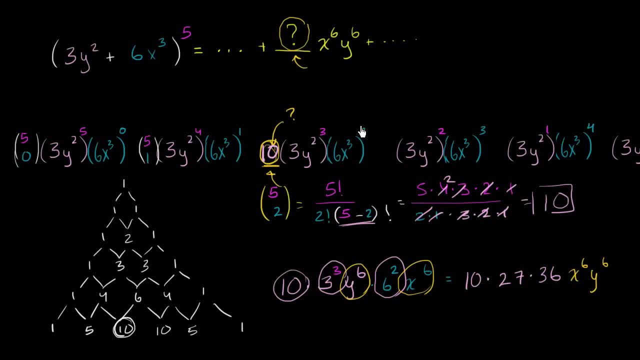 So that's the coefficient. right over here It's going to be 9720 x to the 6th, y to the 6th, 9720 x to the 6th, y to the 6th, and we're done.